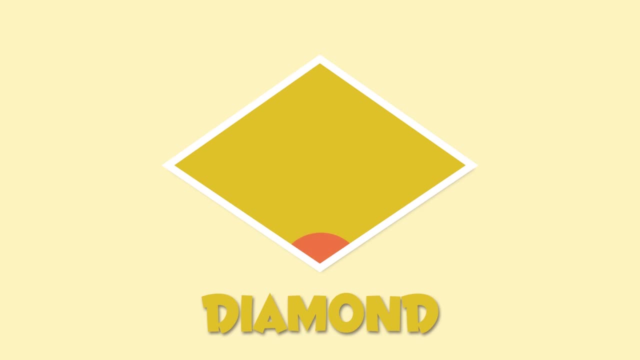 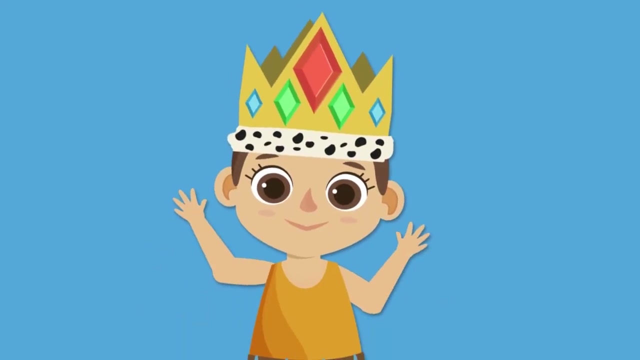 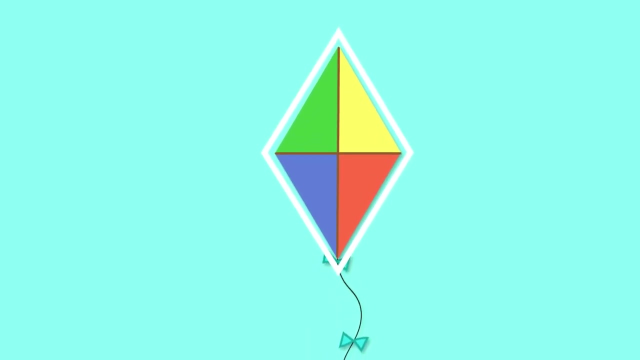 shape. its four sides are identical, but its angles are not, meaning. this one and this one are equal, and so are these two. a diamond looks like the jewel on this crown or like this kite, so this one right here is a pentagon. pentagons have five sides: one, two, three, four and five. 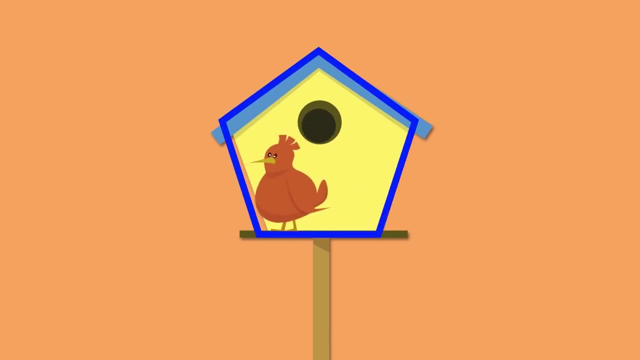 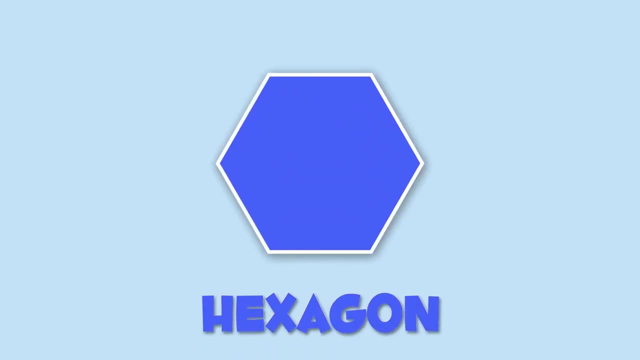 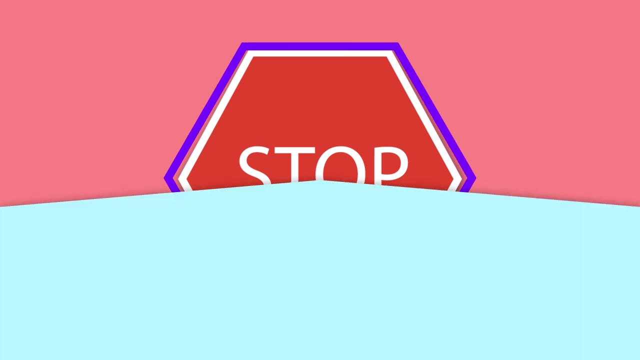 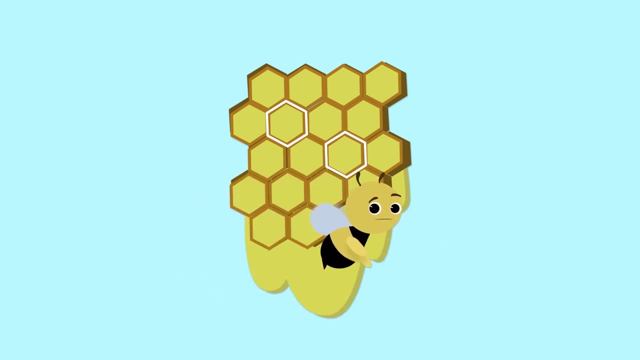 a pentagon looks like this birdhouse or like these football stitches. finally, i'll show you the hexagon. hexagons have six sides. a hexagon is like this stop sign or or like this beehive. we better go now. bees are getting angry. recap circle. 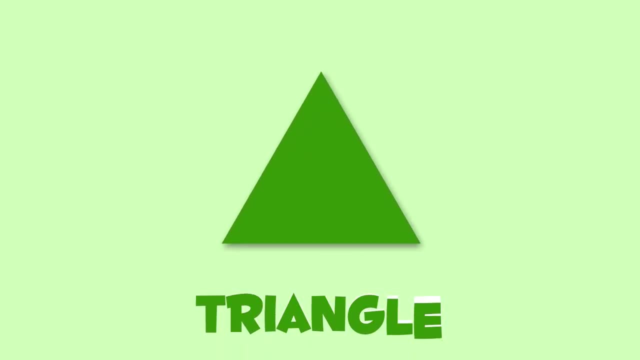 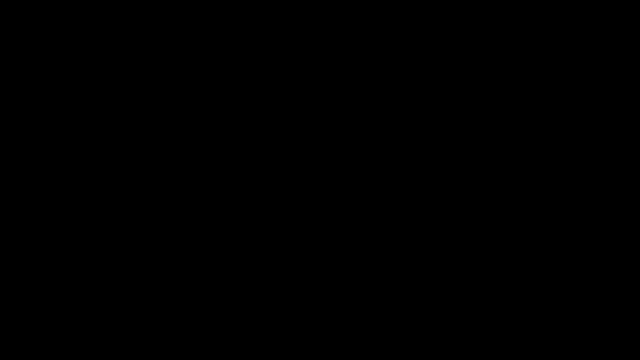 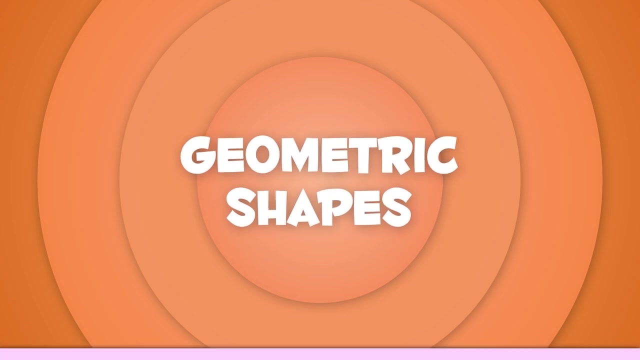 oval triangle, square rectangle, diamonds, pentagon, hexagon, hexagon. now you know everything about playing shapes. well done. today we're going to learn about geometric shapes. do you know how many types are there? here they come. take a guess. what is this? yes, it's a sphere. 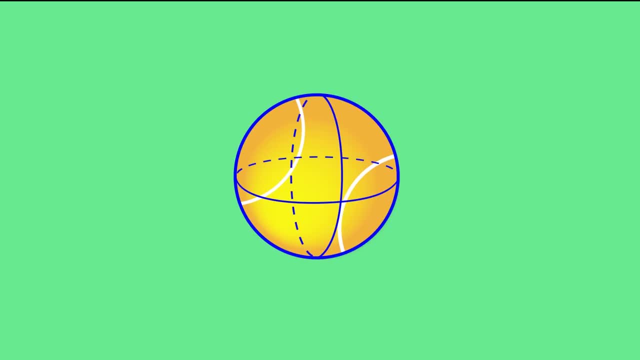 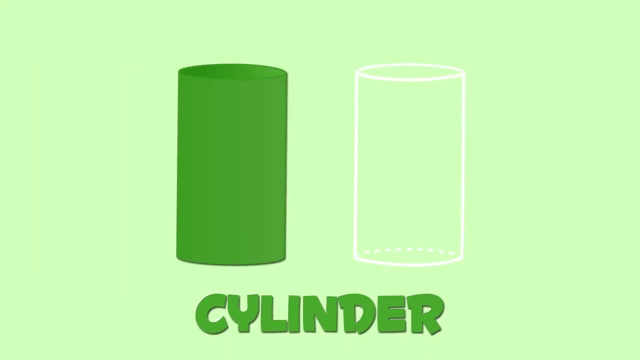 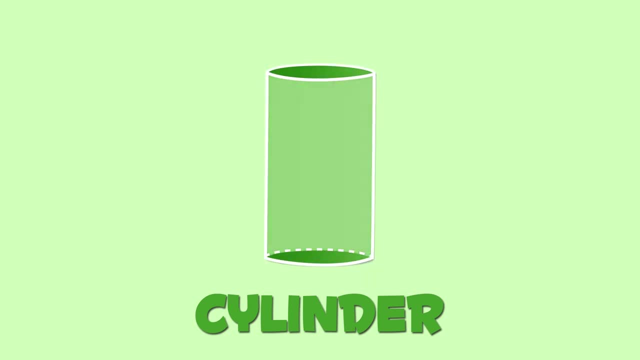 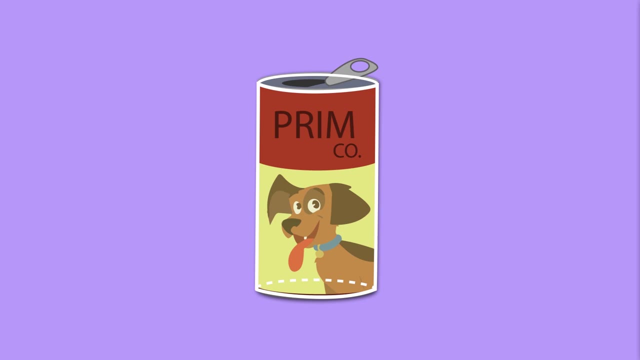 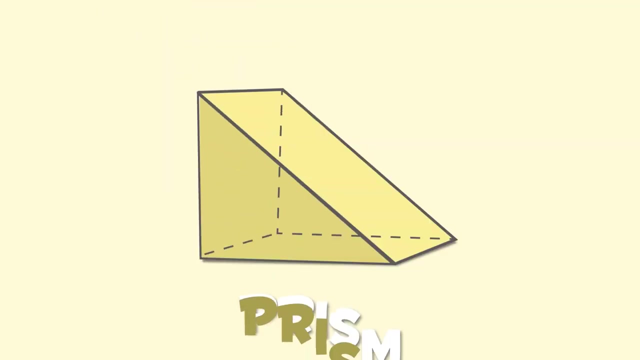 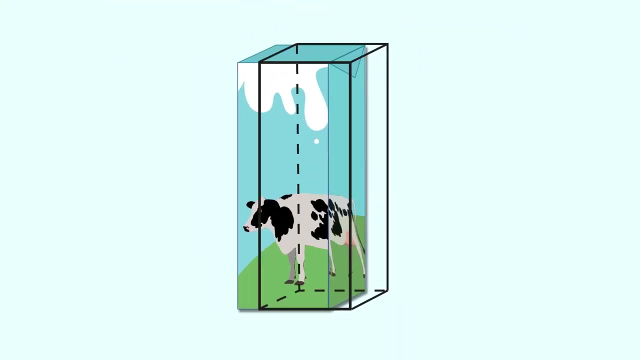 this shape is a cylinder. this shape is a cylinder. this shape is a cylinder. cylinders have two identical flat circular bases. a cylinder is like this can or like this candle. this is a prism. both faces of the prism are identical. there are many types of prisms. this milk carton is a prism. as you can see, both of its faces are identical squares.